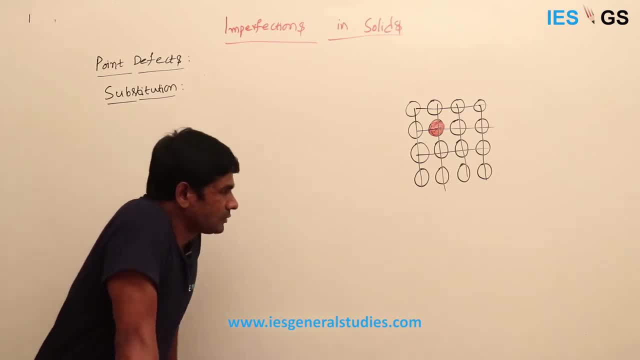 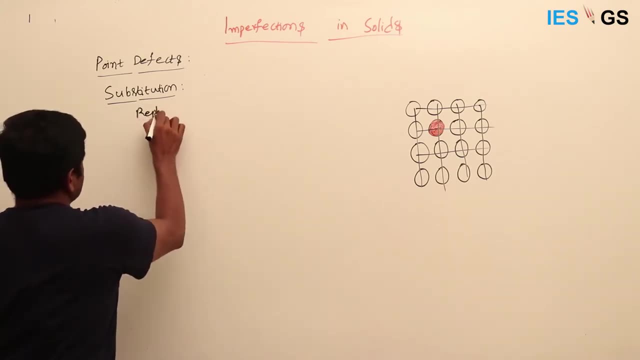 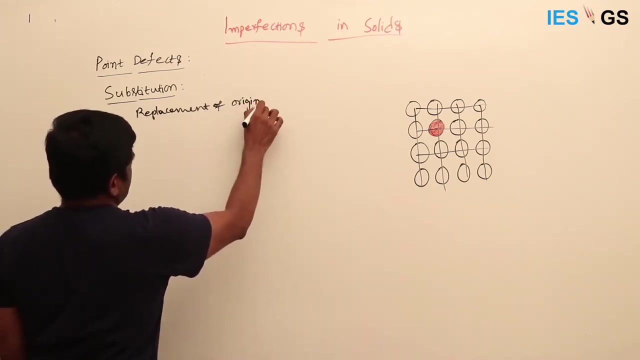 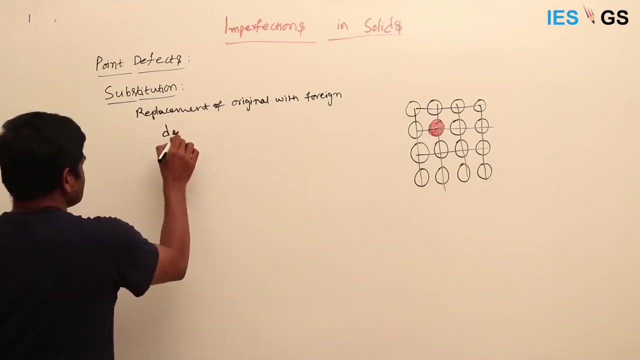 the general things we need to observe here about the conditions. What is that diameter? Okay Here, replacement, Replacement of original or existing with foreign atom- Okay, Foreign atom. And what is the condition here, If you observe generally the diameter of the replacing atom or foreign, let's say, diameter of the foreign. 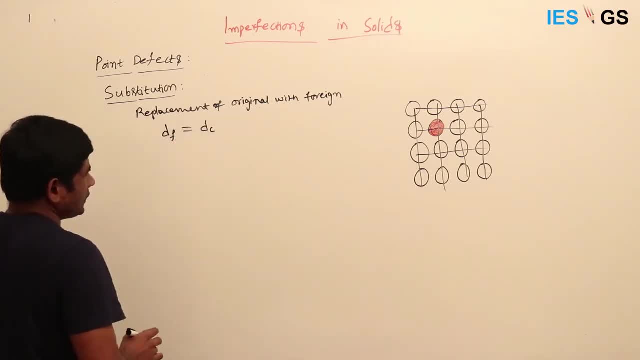 atom is equal to the diameter of the- you know original or the atom, whichever is there already in the cell. Okay, Actually, this is approximately equal. See, sometimes the diameter may be less or sometimes it may be more, But in either case it should not be. 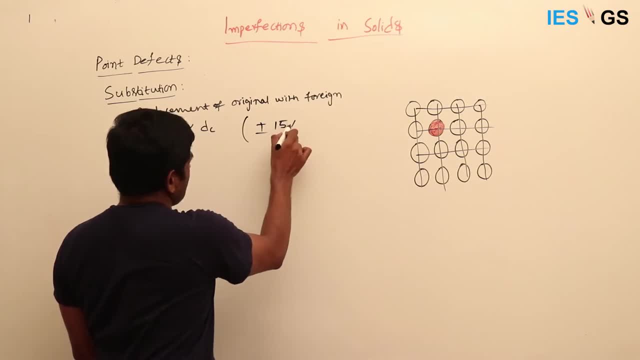 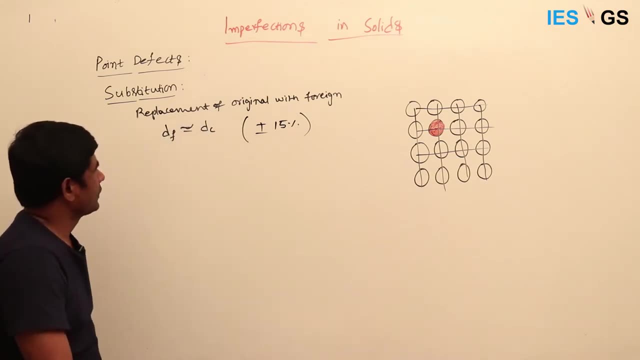 you know, more than or less than 15% of the original diameter. Generally this is the case, Okay. Otherwise the distortion will be very, very high, Okay. And then valency. So valency of the foreign atom should be less than or greater than Here. if you observe, this is simply replacing the 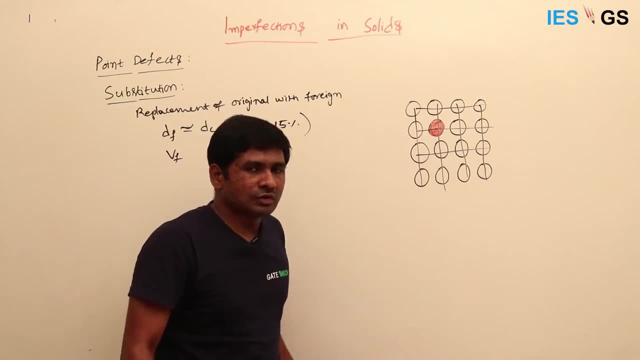 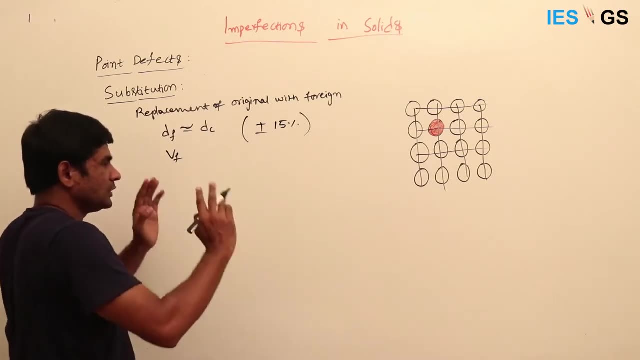 original one. Okay, It is simply replacing the original one. Okay, So this is simply replacing the original one, So the valency should be equal to the original one. Okay, When I say should be, don't think it is only should be equal to. Actually, it it it equal generally, it is equal to the. 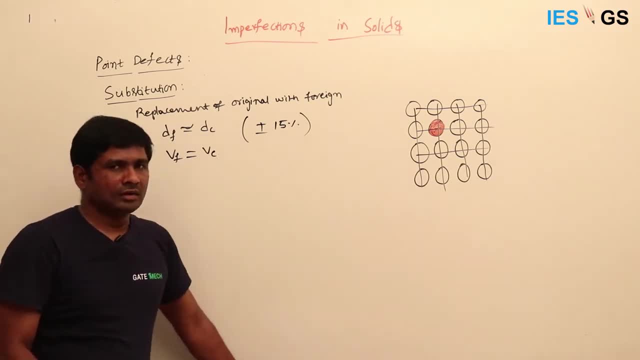 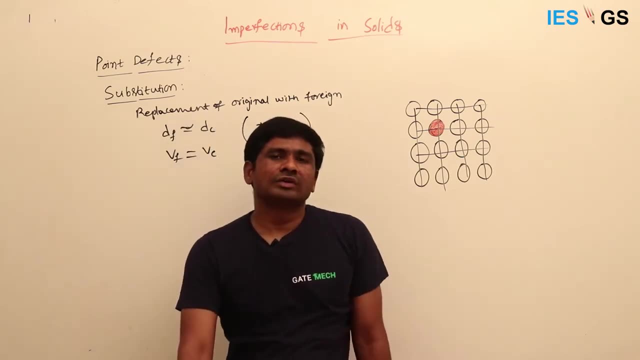 original atom. Sometimes, you know either, you can insert some atom which is more than that. For example, here, some of the time we will insert a silicon into the gallium atom. So silicon is having a you know not equal number of. you know not equal number of. you know not equal number of. 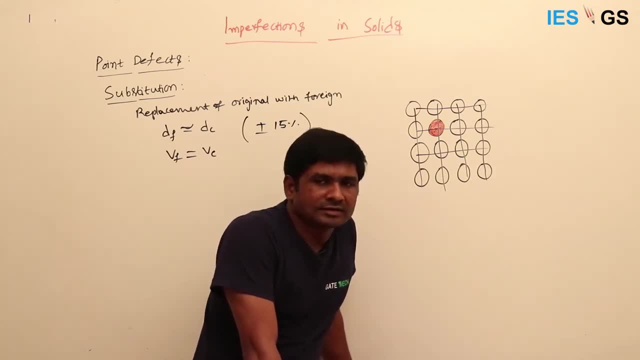 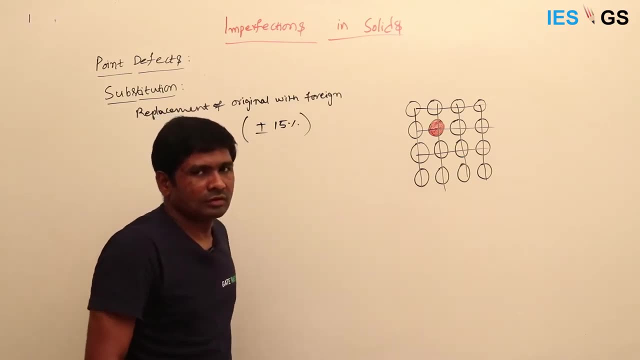 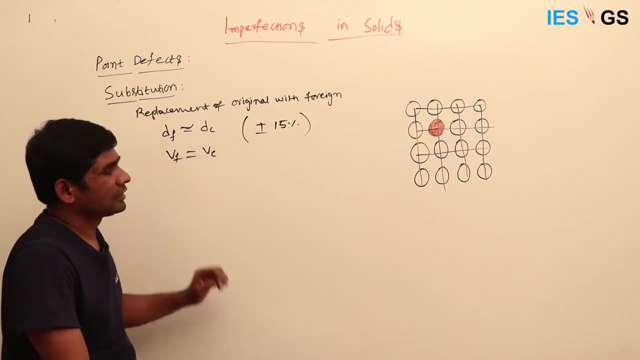 you know, electrons as that of gallium. Okay, There is a difference, But the difference is not that much, Only one. Okay, So here, generally vacancy will be, you know, equal. Here, in this case, generally vacancy, sorry, valency, not vacancy, Sorry, Valency will be equal and diameter. 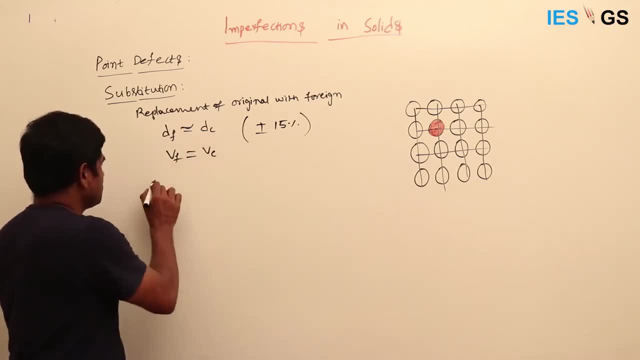 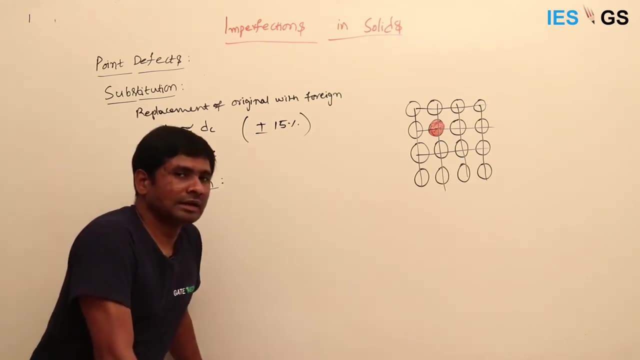 also equal. Okay, And coming to the strength. strength, is there any change in the number of bonds here formed? No, Why? Because we are simply replacing the original one and you know it is still maintaining the same number of bonds that it is having previously. So strength you. 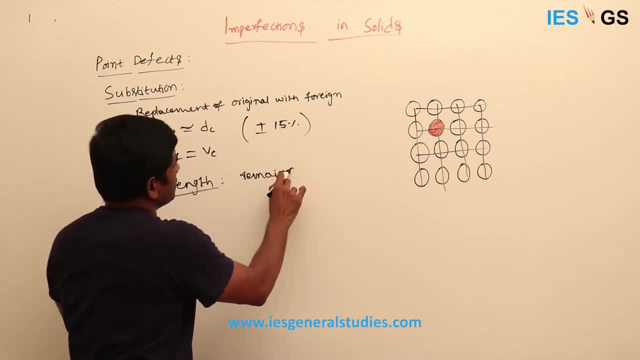 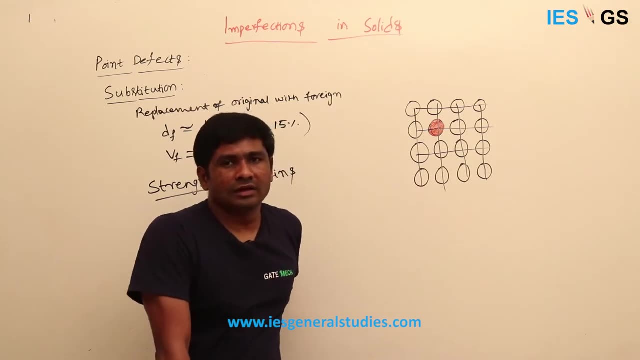 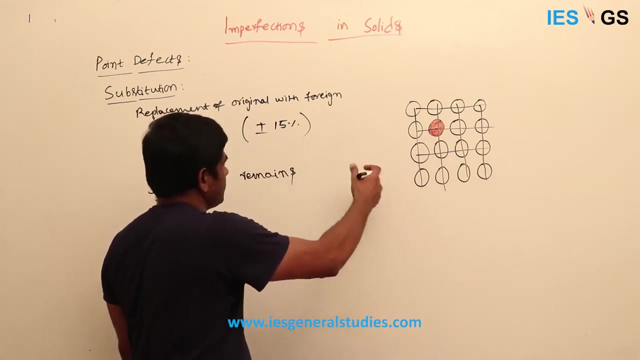 know, remains the same, Remains. of course there is some small changes. Okay, Why? Because the atom is changing. There is a difference in the, the amount of attraction between these atoms, amount of, you know, bond between these atoms. Okay, Then there will be very, very minute change, But 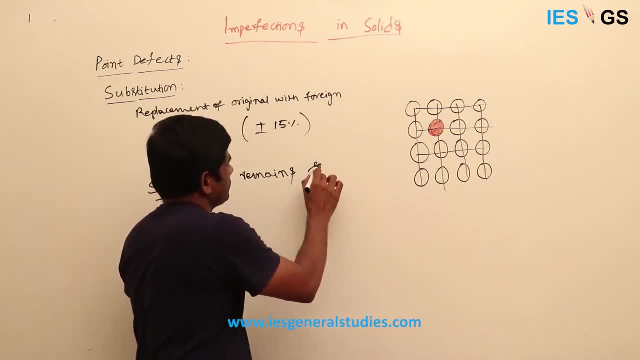 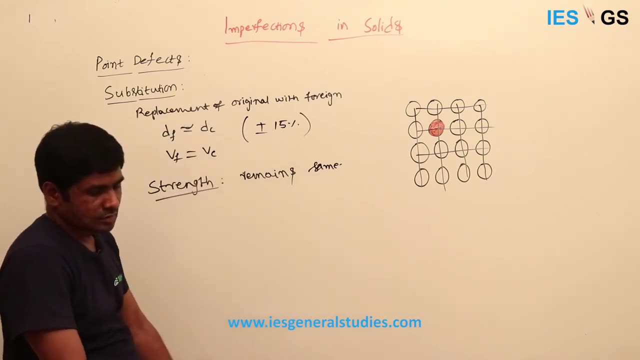 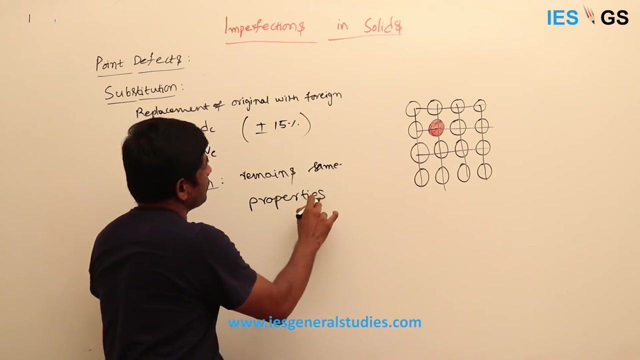 we can say: remains same, Okay, Not affected. So here what would be the example? We see strength. strength not change. The strength of strength of the material may not change, But the properties may change. here if you observe Properties, Even in the previous case also properties changed. Why? Because in 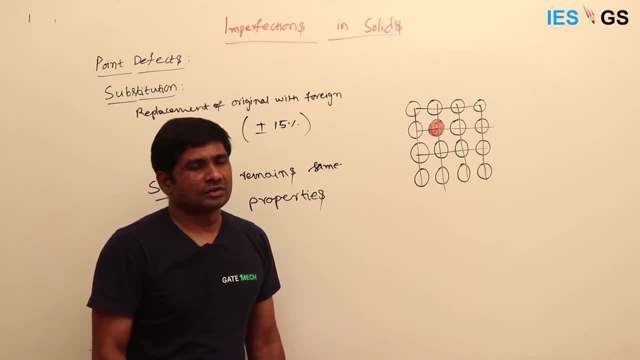 the substitution and vacancy. the number of atoms are changing. So there is a property, Especially in the interstitial atom. other new atom is coming and sitting, So that properties are also changing Here also, even though the strength is remained same, properties are changing. Why 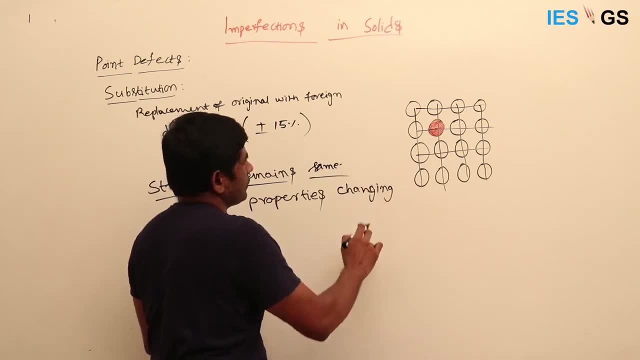 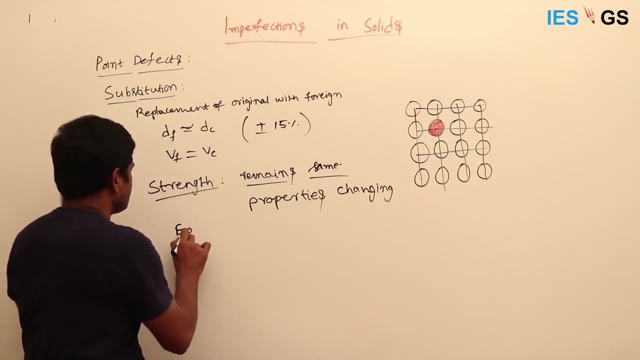 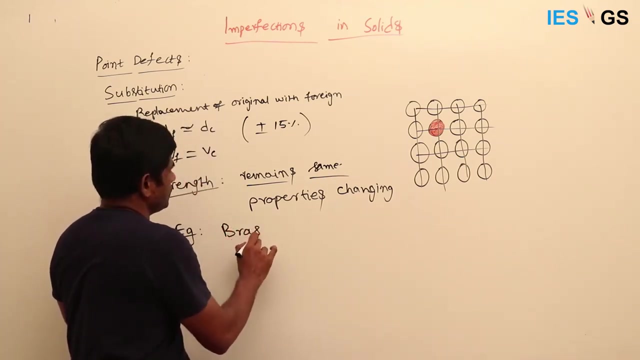 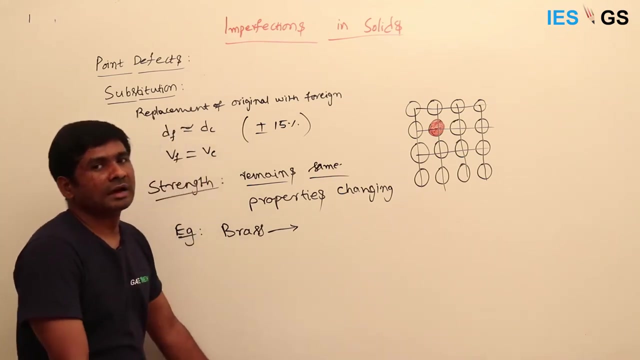 Because there is a new atom here, you know from the original atom. Okay, And here, what is the example? for this Example is: for example, you can take brass. Okay, You can take brass. What is the brass here? See, you remember brass, This is important. Brass, bronze, these metals, I, I will. 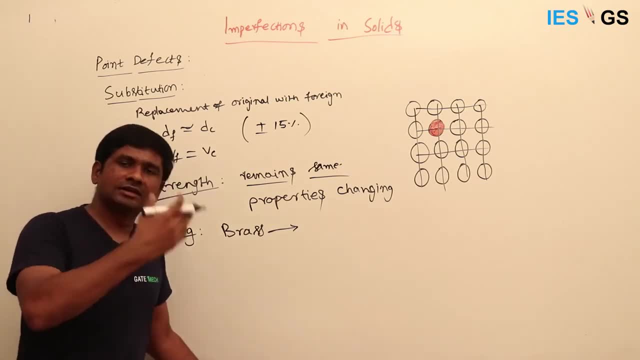 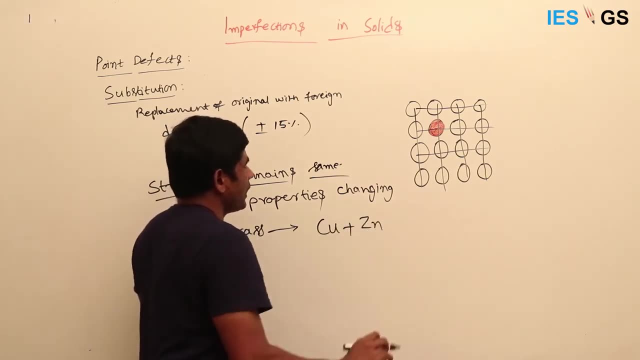 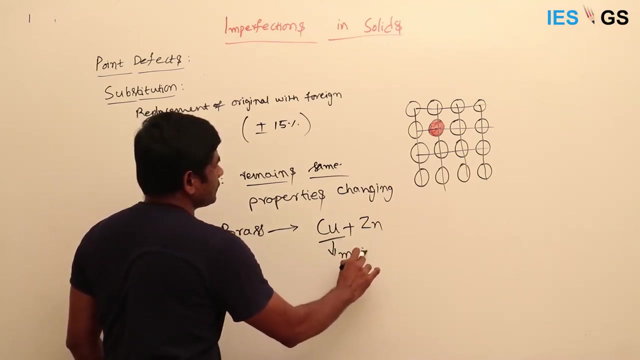 deal. you know separate topic for that. I will take all the general materials and I will explain. So brass is a combination of copper plus zinc. If you add zinc to the copper actually here out of these, this is the main component. Copper is the main component here. Okay, So if you add 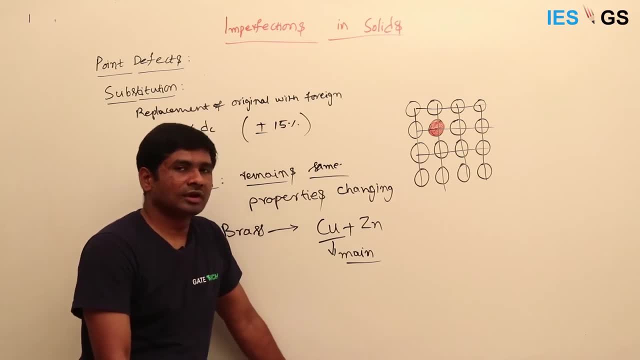 zinc to the copper. then what happens? The copper strength, the copper strength, the copper strength will be increased, Its strength will be increased. Of course, even the strength is increased. it is not more than the steel, Okay, So its strength will be increased. So that is why we 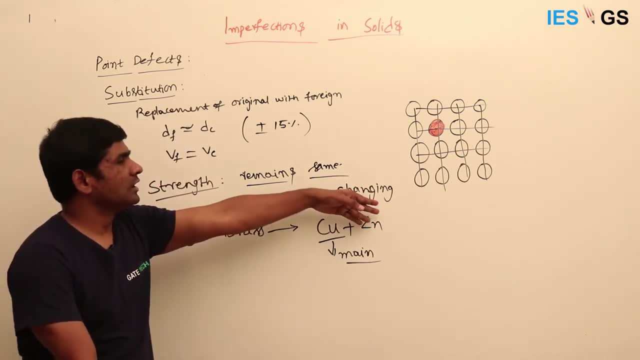 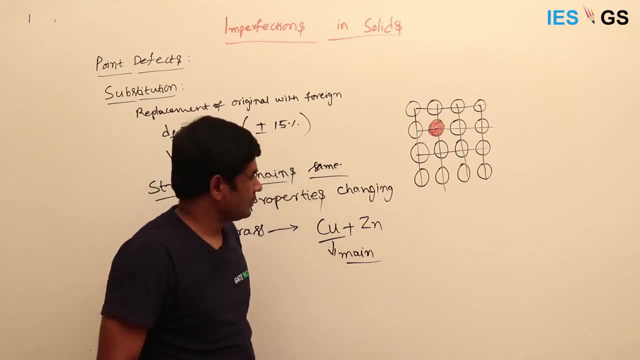 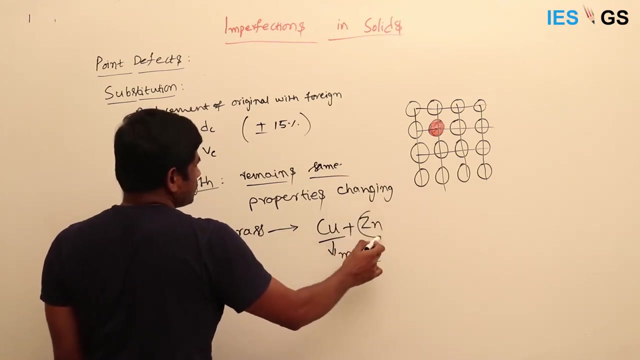 are adding zinc to the copper here. See, this is very ancient invention, From the old and very ancient days. we have a bronze and a brass. you know articles, artifacts. So here what is happening When adding a zinc, then it is replacing some of the atoms of a copper. 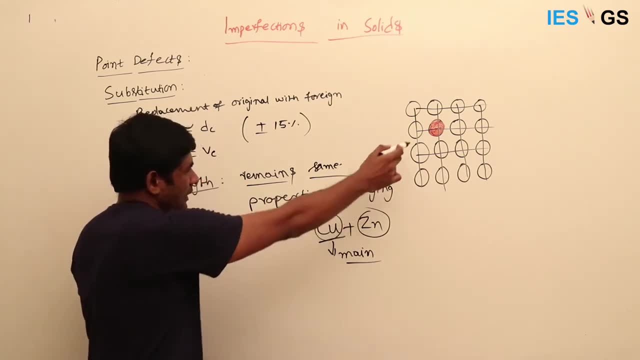 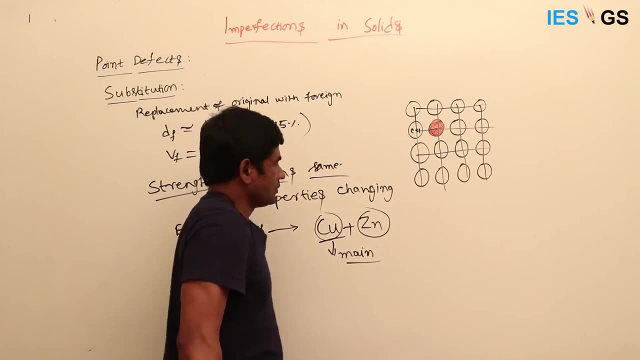 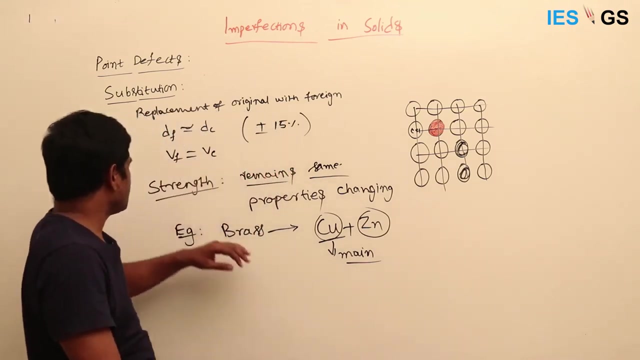 okay, it is replacing. for example like this: these are all copper, let's say these are copper. so some of the places it is replacing with the zinc, okay, maybe here one under here, one here, one more zinc, like that. you know, some of the places is there is a replacing, so that is called as the substitution and here: 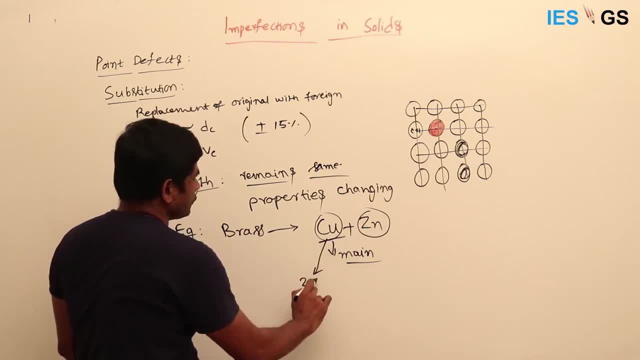 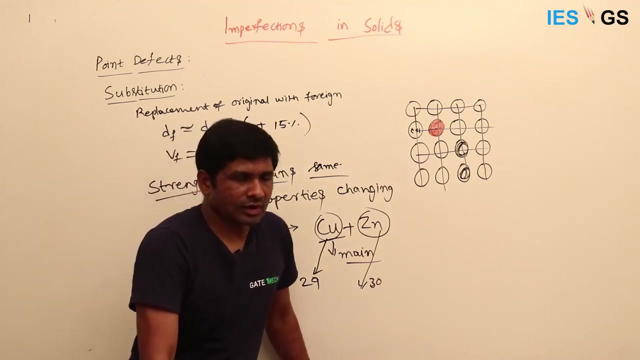 if you observe, the copper atomic number is 29 and zinc is 30. so these are very nearer, so that we can say the number of you know, electrons are very nearer to one another, so that the size of the atom also very nearer, okay, very, very nearer to this. so here, that is why we can easily replace with the in zinc. 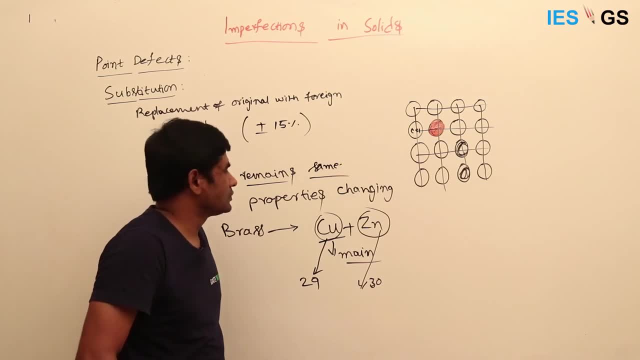 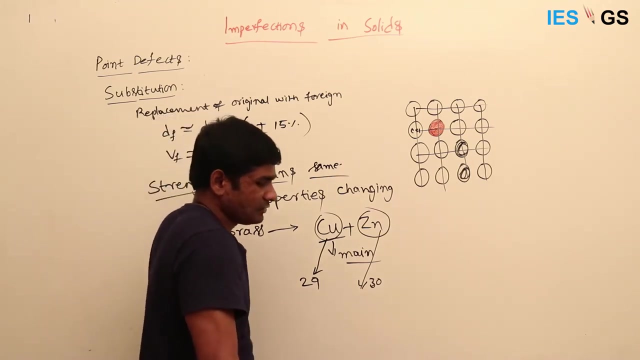 in our car, parotid can be replaced with the zinc. here, on a valency, of course there is a difference in valency, but still it is a, you know can go, and here okay, we, we, we talking about advantages, always okay, even in the interstitial defect, we said that, you know. 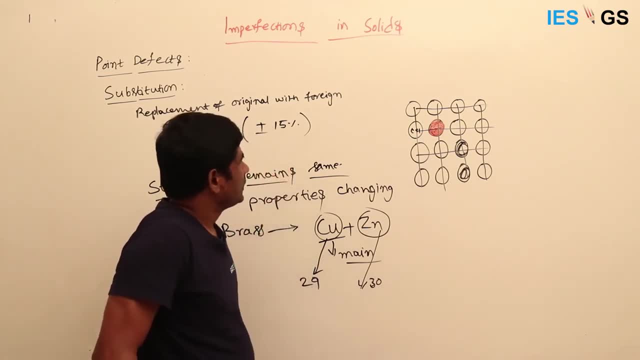 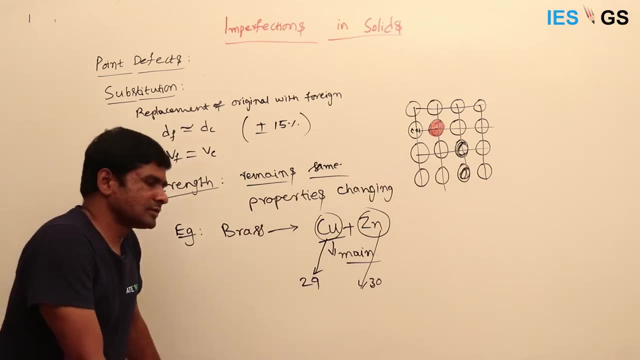 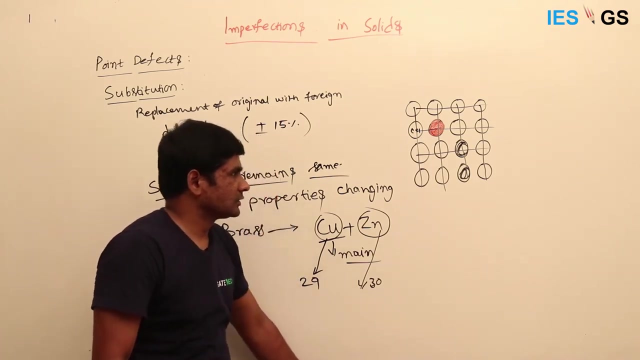 steel is formed because of that, and here also, here also, we are saying bronze will be found, you know with this. but where is the actual concern that is happening and why we are treating them as a defect? why we are treating them as a defect. see, if you observe, in case of vacancy, it is very 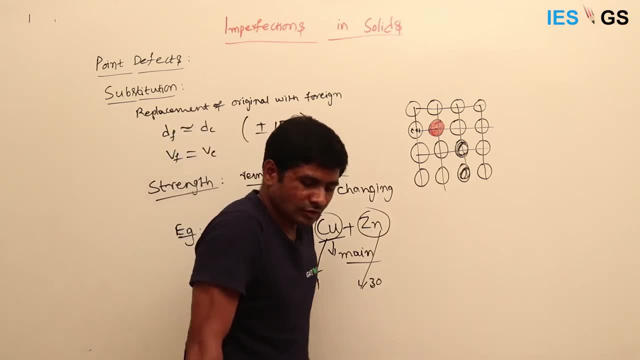 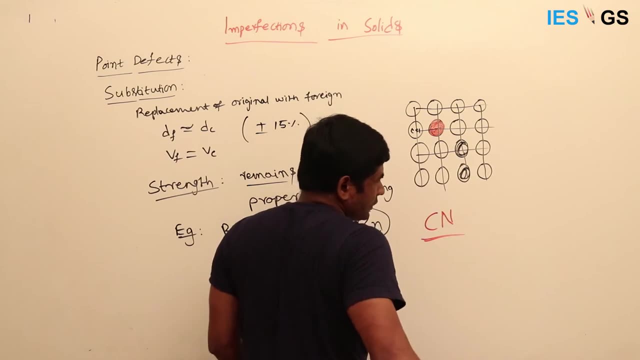 evident. okay, no need to worry. but in other cases also, you can observe that the coordination number is changing. here, the coordination number changing. what is the coordination number if you consider any atom? okay, so how many nearest atoms are there? or what you know, the particular atom, whichever? 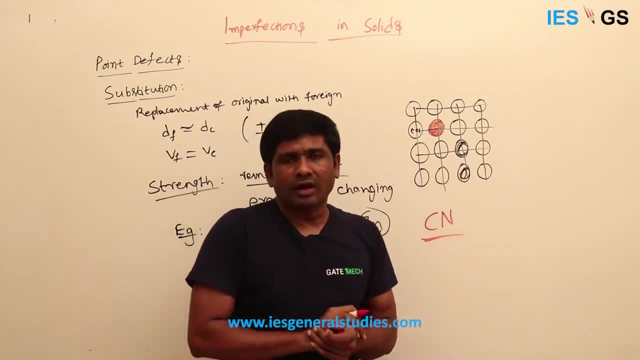 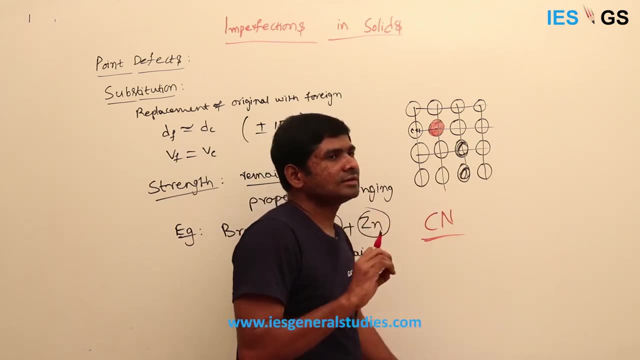 you consider with how many nearest atom it is forming the bond. in other words, you know if the how many atoms it is in the touch. okay, so in the previous vacancy and interstitial it is evident that you know coordination number is clearly changing. even here. in this case also there is 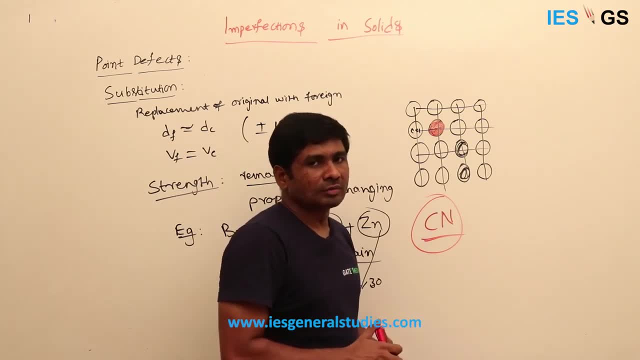 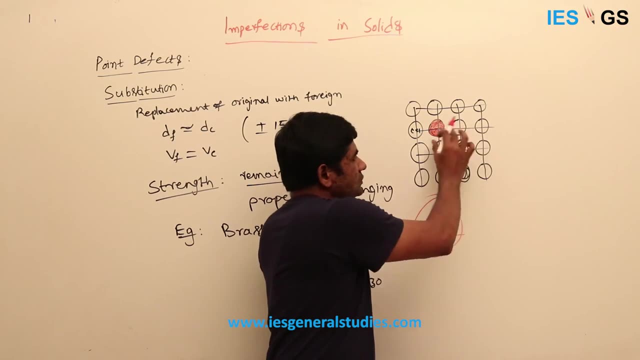 a slight change in the coordination number. why? because it is also depending on the size of the atoms, the coordination number. okay, for example, if you put a very small size of atom which is not touching the atoms, other atoms, then you can say that the coordination number is affected here.